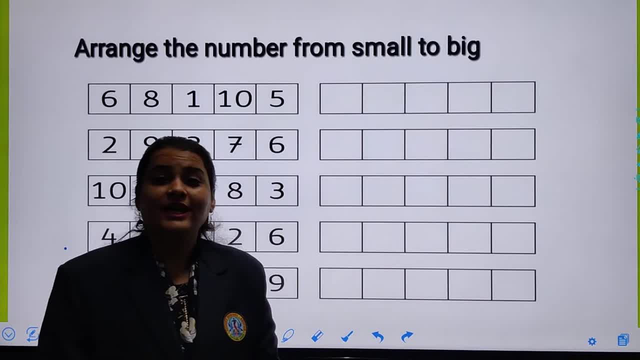 Okay, For that, what we have to do? For that we have to do road counting. Okay, Here, what numbers are there? There are numbers between 1 to 10, right? Yes, Here we have numbers from 1 to 10.. 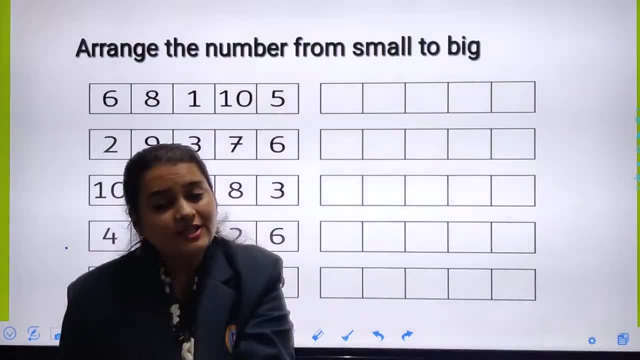 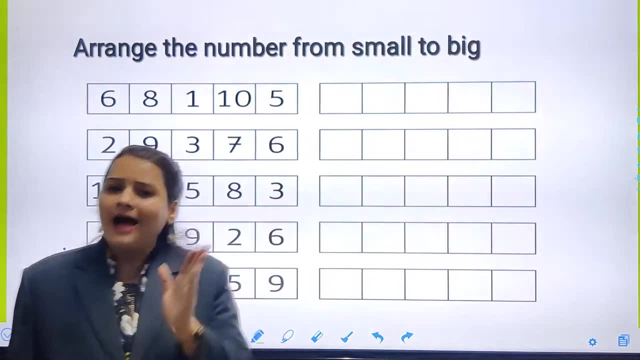 So we will do road counting from number 1 to 10.. What we will do: We will do road counting from number 1 to 10.. Okay, And the numbers which come while doing road counting, we will arrange the numbers given here. 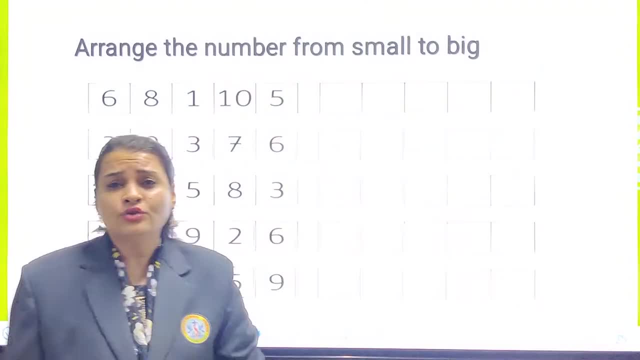 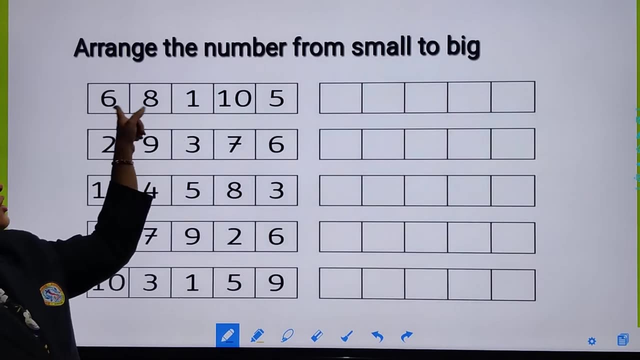 Okay, Okay, I will show you. So first we will do road counting. Number 1. Number 2. Number 1.. Okay, So can you see here Number 1. Number 1: is that Yes? 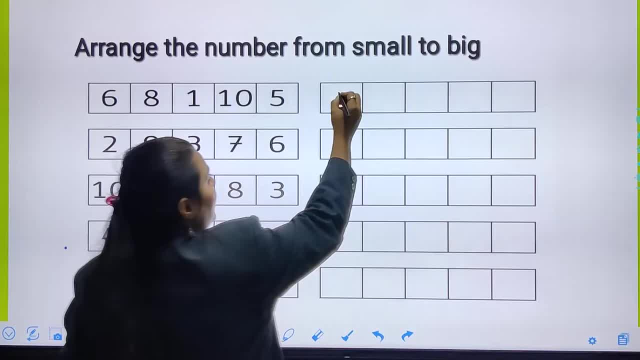 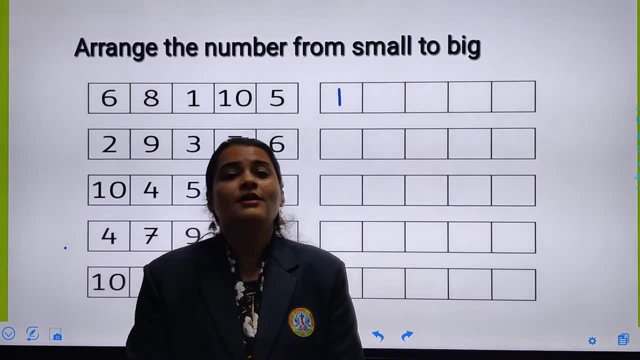 Yes, Number 1. is that Okay? So first I will write number 1.. Then which number will come After number 1?? Yes, Number 2 will come, But number 2 is here in this line No. 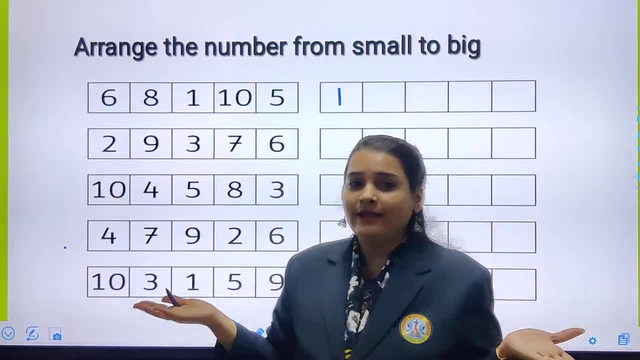 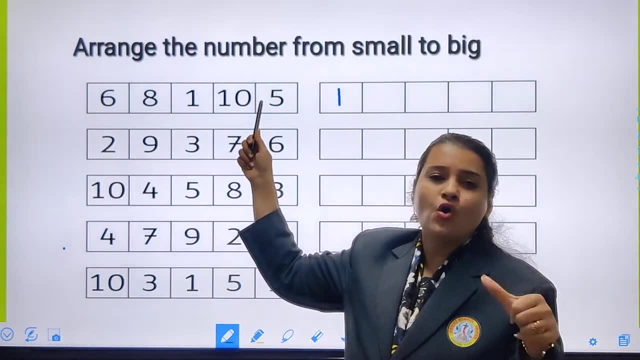 No, number 2.. So we don't have to write number 2.. Okay, Yes, Then which number will come? Number 3. Number 3 is here. No, Number 3 is not there, So we don't have to write. 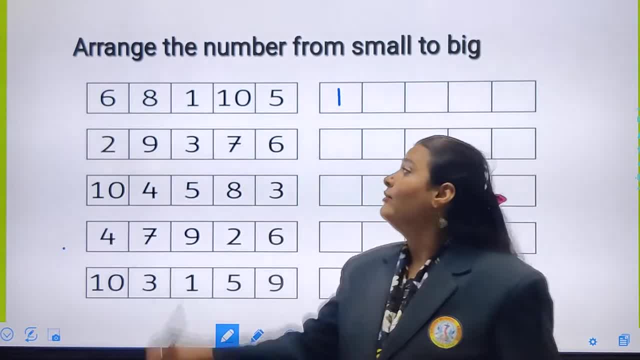 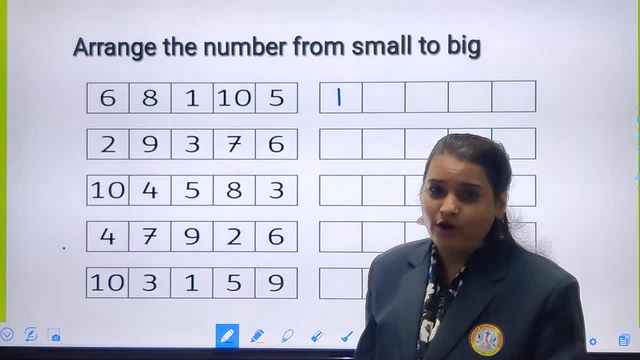 Okay, Then number 4 will come. Number 4 is here in this line. No, That is no number 4.. So we don't have to write number 4 also. Then which number will come? Number 5.. 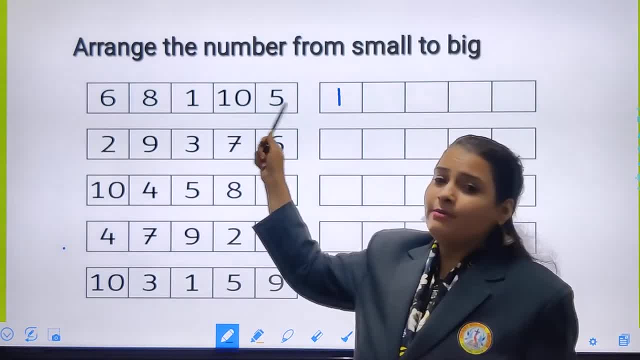 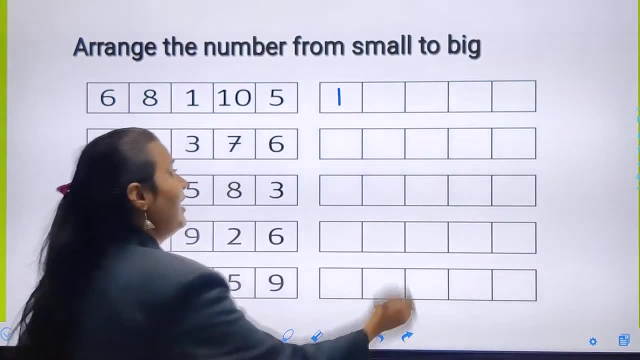 Number 5.. Yes, Here we have number 5 in this line. Yes, Here we have number 5.. Number 5 in this line. So I will write number 5 over here. I will write number 5.. Yes, 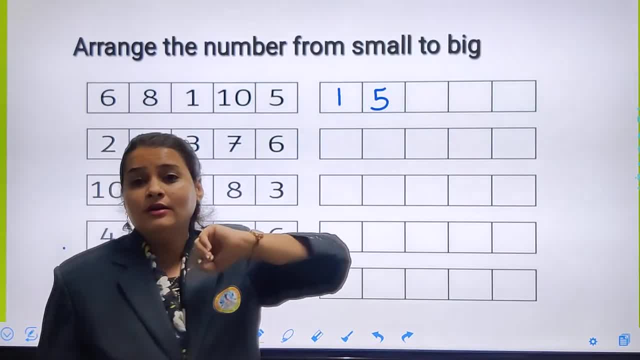 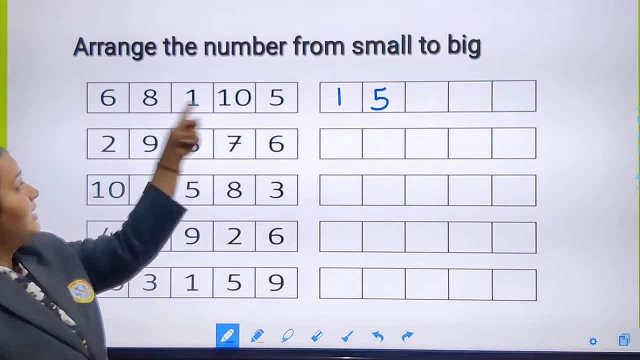 Yes, Then what I have to write in this next block? Yes, Okay, So which number will come after number 5? Number 6.. Number 6 is there? Yes, Here we have number 6 also, So I will write number 6.. 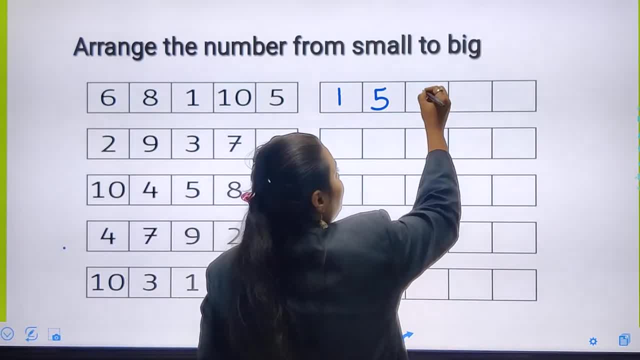 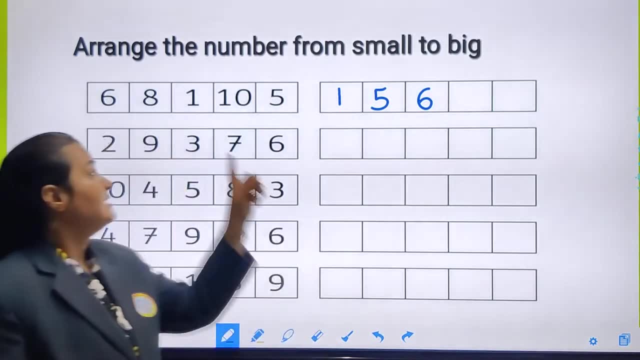 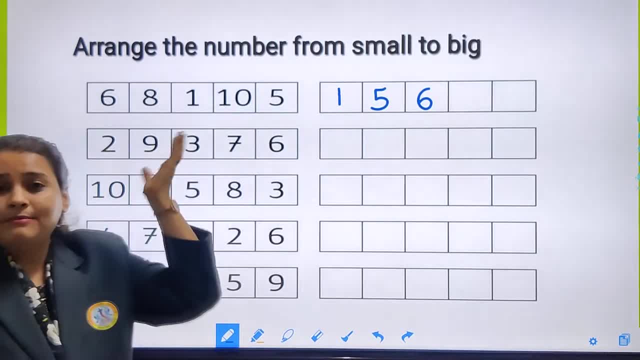 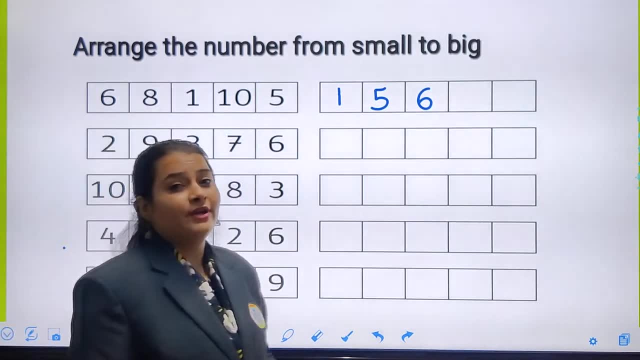 No 7 number is there, So I will not write number 7.. Yes, Then I have to write number 8, because which number will come after number 7? Number 8 will come. Yes, And here we all can see number 8 also. 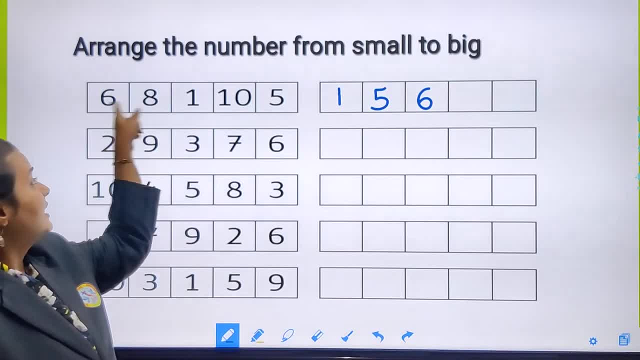 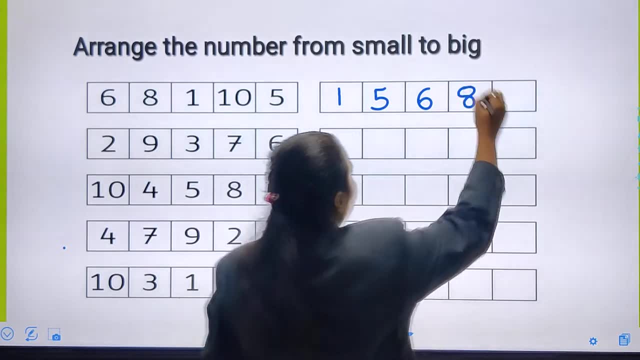 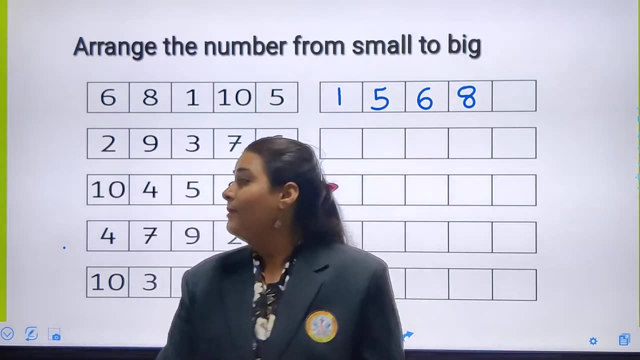 Yes, So I have to write number 8 over here. Then which number will come after number 7? Number 4.. And which number will come after number 8? 9.. Number 9 will come, Yes, But is there a number 9?? 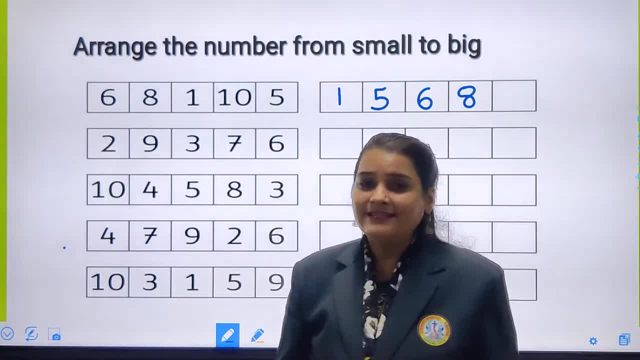 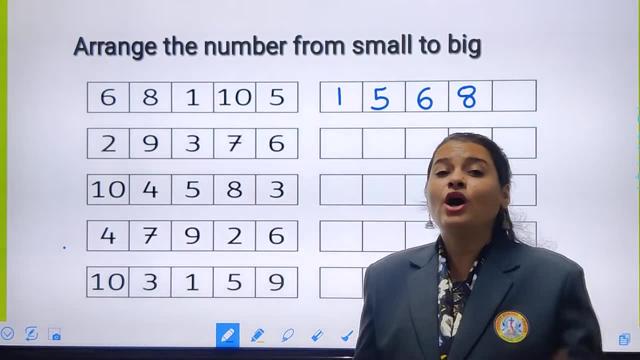 No, Number 9 is not there. Yes, So I will not write number 9.. Yes, Okay, So which number will come after number 9? 1, 0, 10.. 1, 0, 10 will come. 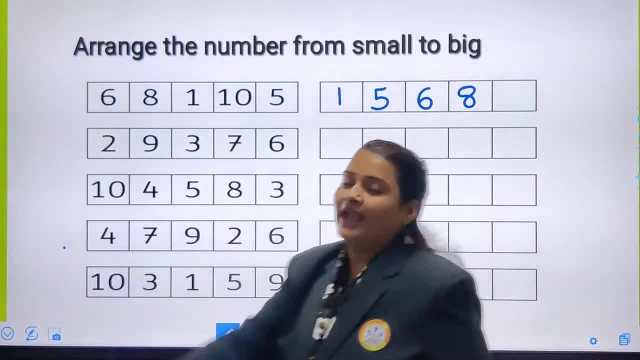 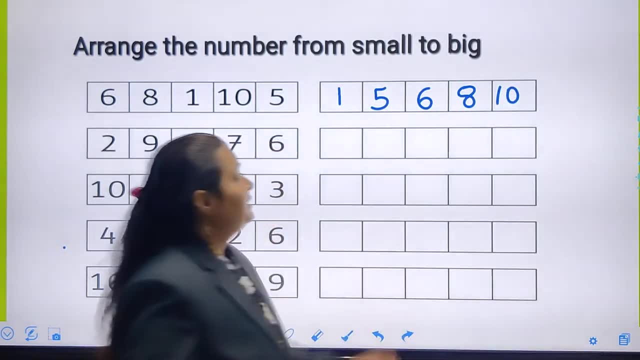 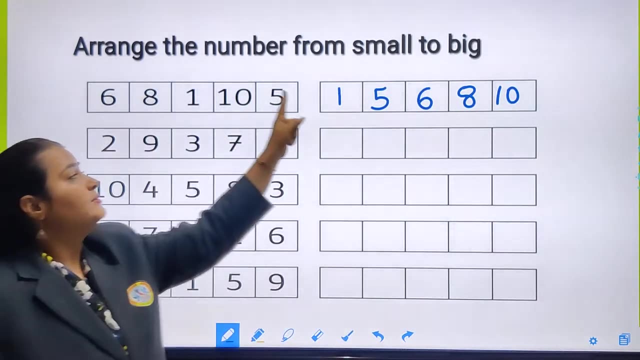 Here we have number 10.. Yes, Okay, So I have to write number 10 in this last block. So this is small number and this one is big number, Right, These numbers are given Out of them. this is small and this is big. 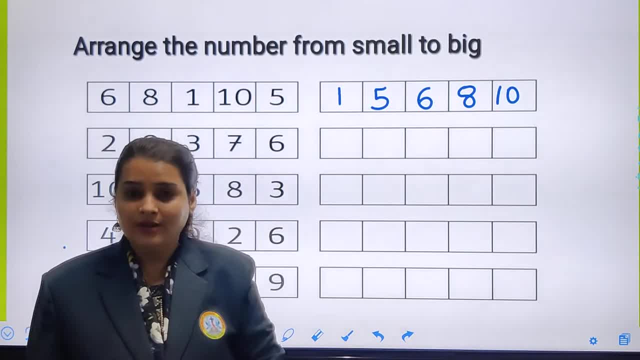 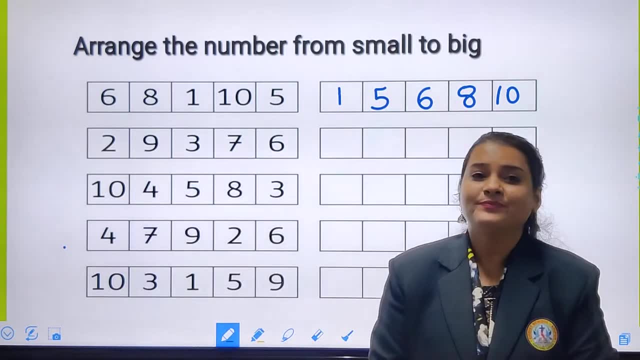 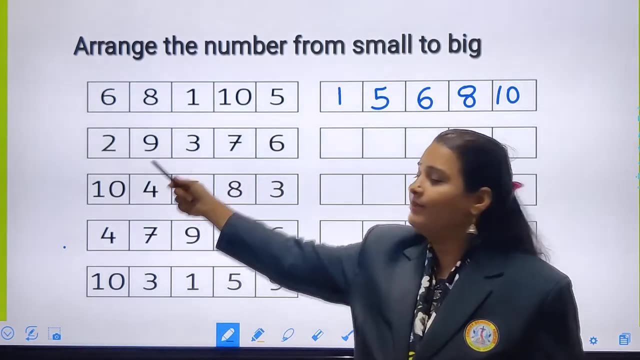 And we have arranged from small to big. Okay, We arranged these numbers from small to big. Understood, Yes, Yes, Yes. So now here we have one more line. Okay, Some more numbers are given in this line, Okay. 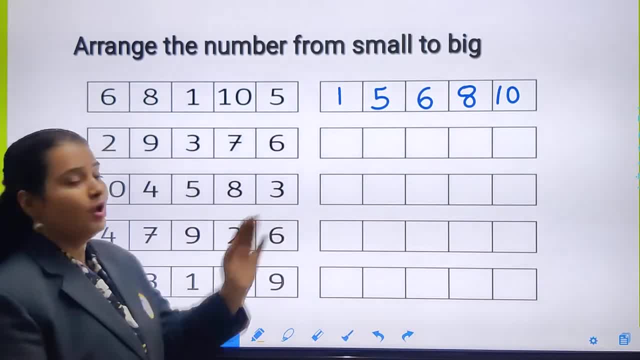 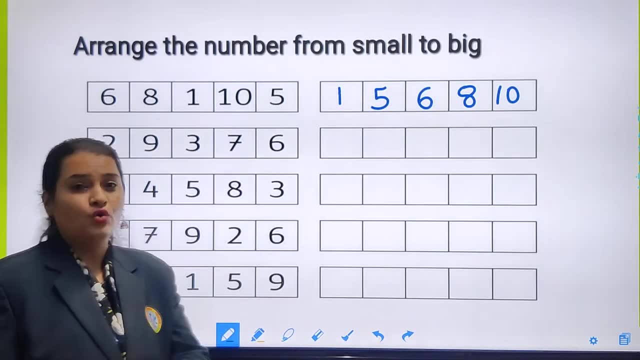 So shall we arrange these numbers? Yes, From small to big. Yes, So first I will count from number 1.. 1. Then 2. You can see number 2 over here. Yes, So I will write number 2.. 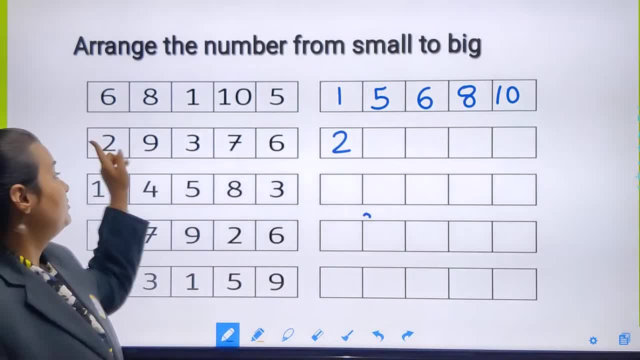 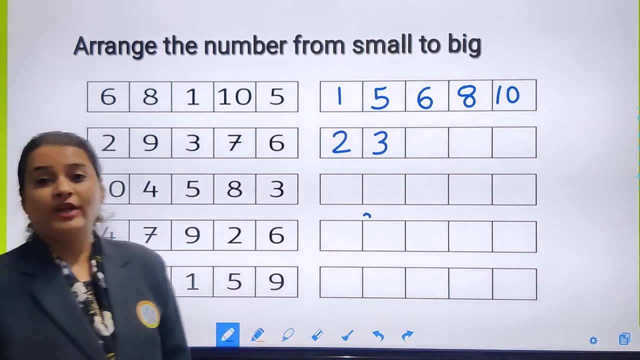 Then which number will come? Number 3.. Number 3 is there. Yes, Yes, So I will write number 3 over here. Then which number will come? 3,, 4,, 5.. Then, after 5, which number will come?